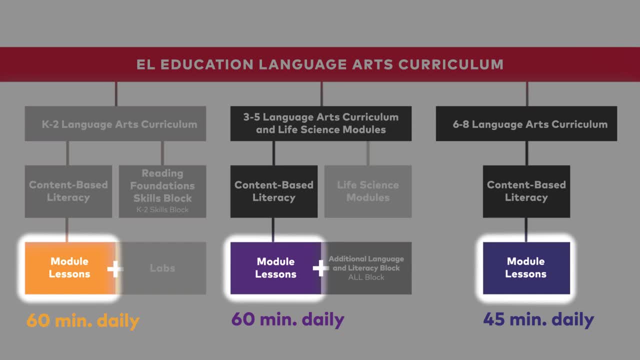 of the college and career-ready standards for reading, writing, speaking and listening. Graduate-level lessons include a quality of life program, a library, up-to-date curriculum and a complete, barrier-free curriculum With each graduate in college. in turn, the curriculum 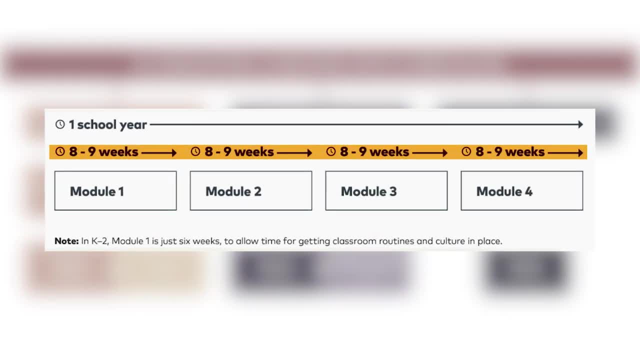 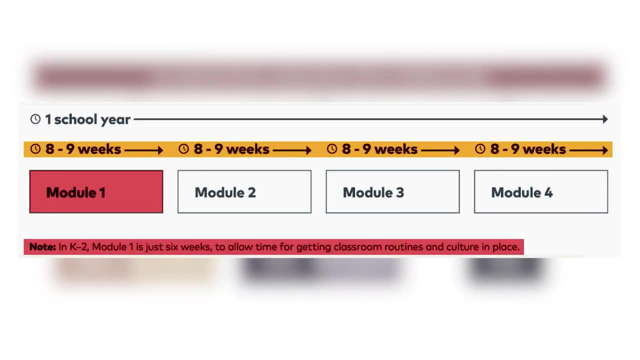 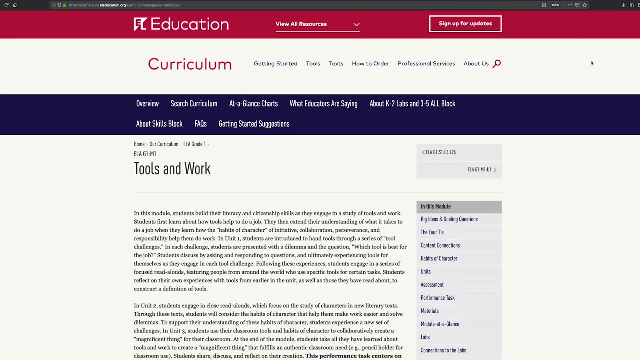 Each module comprises eight weeks of content-based instruction, with the exception of the first module in grades K through 2, which is just six weeks long to provide the time to establish routines that ensure success throughout these formative learning years, Every module has been designed to have a 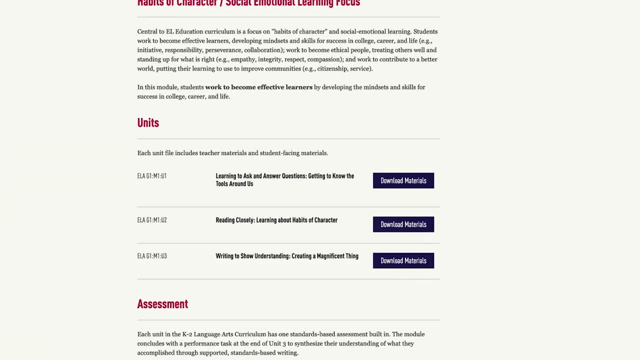 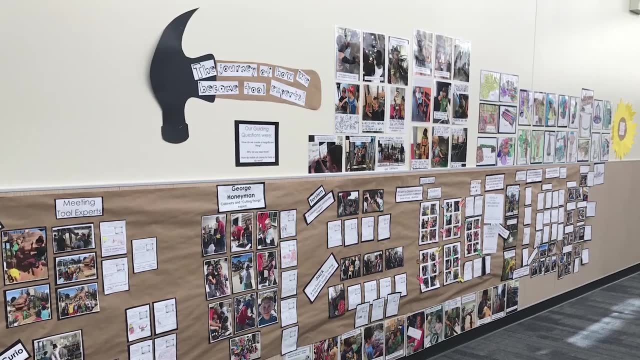 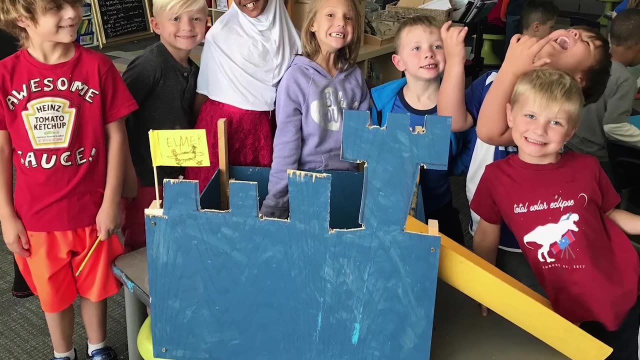 compelling story or conceptual through line that unfolds over the course of three units. Grade 1: module 1 revolves around reading and writing about tools, including the anchor text- the most magnificent thing For the performance task. at the end of the module, students design, build and write about their own. 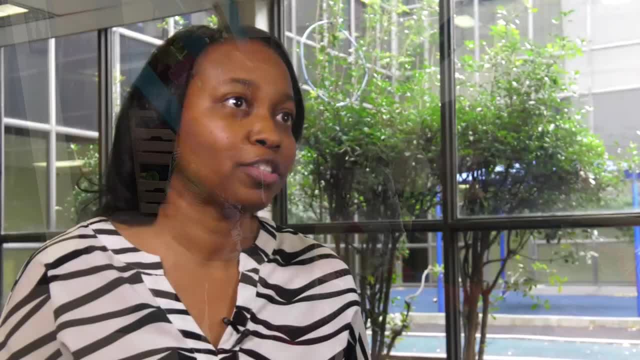 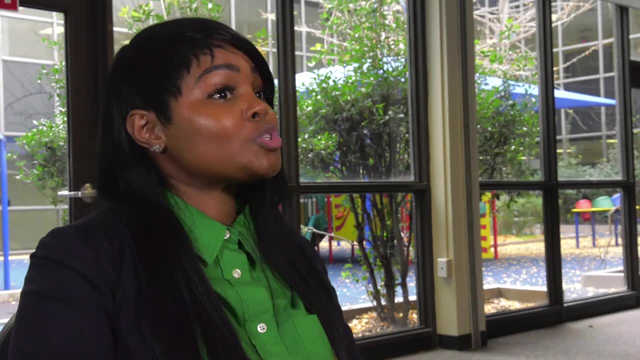 magnificent thing for classroom use. Children had to use those habits of character and they had to build a magnificent thing, something that could be used within the community. How can you show initiative with starting to build your most magnificent thing, and then how can you collaborate? They're able to. 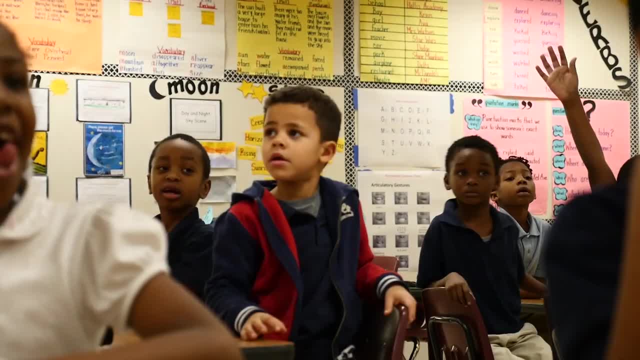 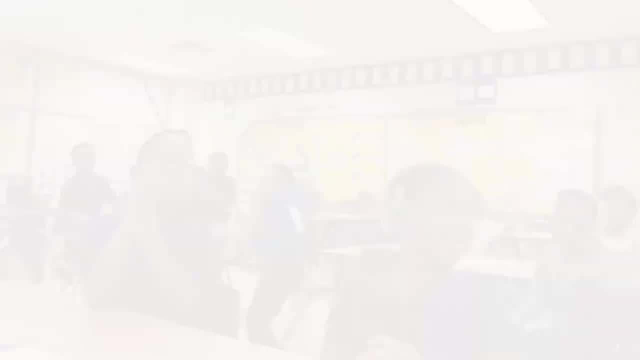 actually read it and hear about it in the text. but it doesn't have to be the most magnificent thing, It has to be the most impressive thing. It doesn't stop there. Now they have to apply it. One group did a mailbox. one group did a sight word: mobile. Unit 1 of every module engages 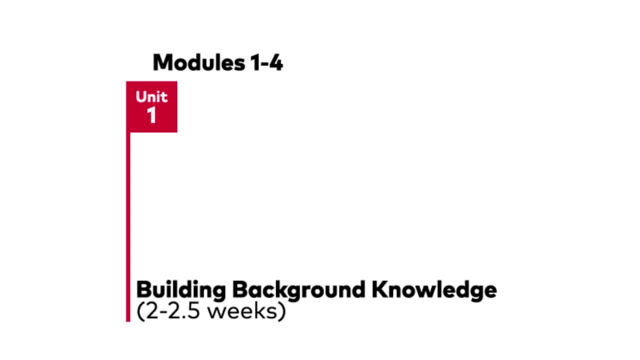 students in the topic and helps them build background knowledge, vocabulary and academic language. Then in unit 2, students dig deeper into the topic, exploring additional texts of varied text types. Unit 3 requires students to apply their learning to create an authentic product in the performance. 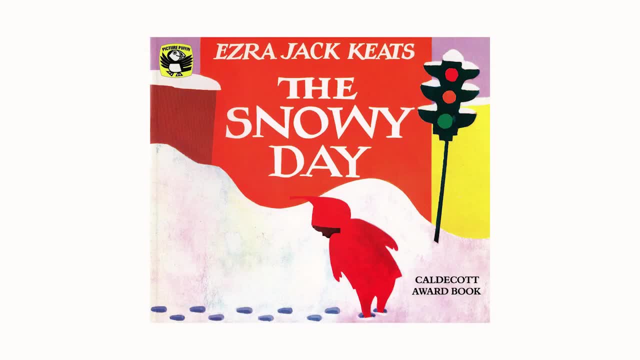 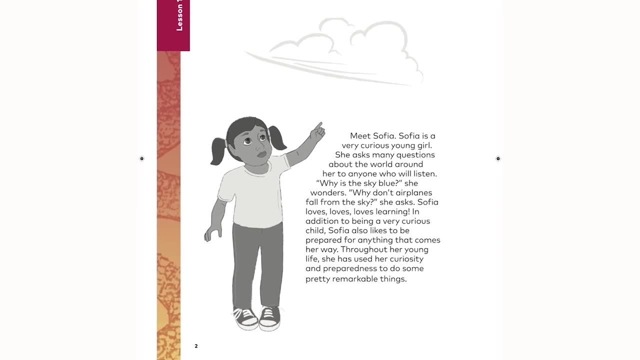 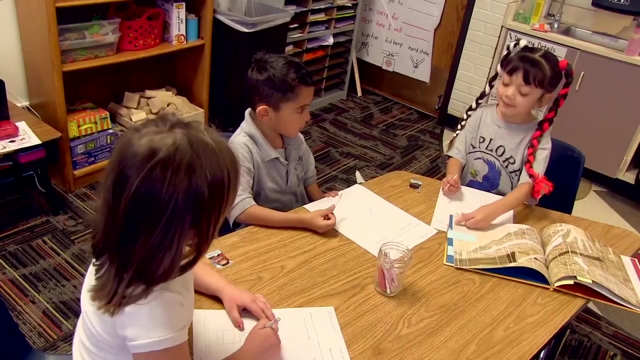 task. The sequence of the text in a module unfolds logically. Students engage in a topic while building their knowledge and skills. Through the content, students are guided towards mastery of the standards taught and assessed in that module. The books on the tables, all of them, were open. The kids were finding 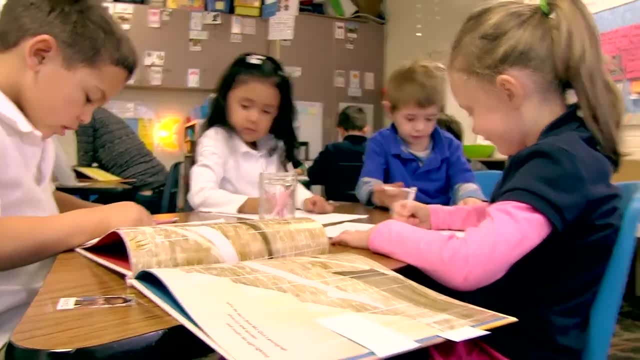 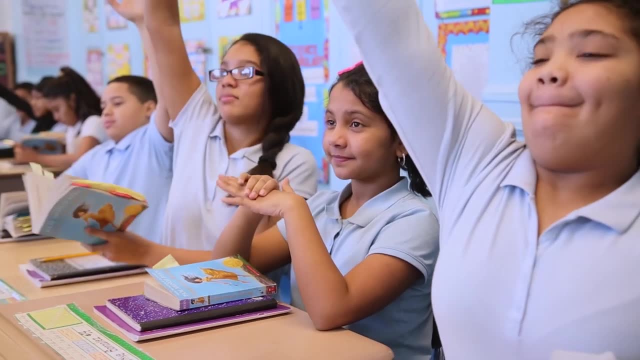 pages and looking at pictures and using words directly out of the book. In grade 5 module 1, students begin the module by reading the anchor text Esperanza Rising to engage the students in the topic. In grade 5 module 1, students begin the module by reading the anchor text Esperanza Rising to engage the 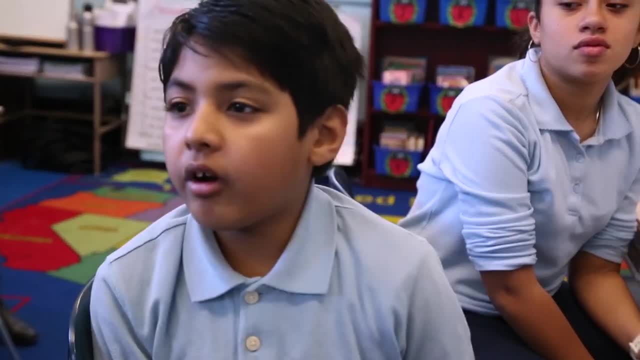 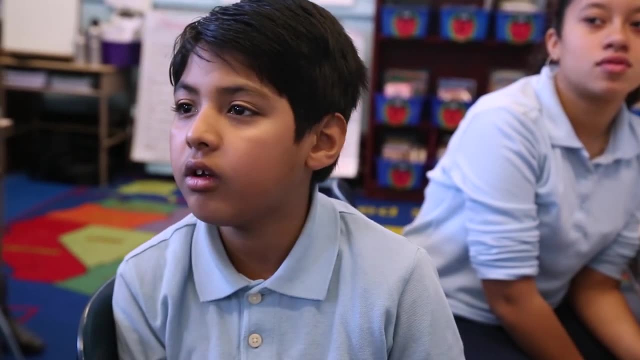 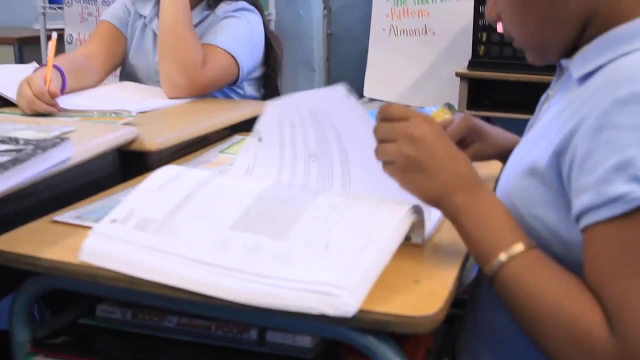 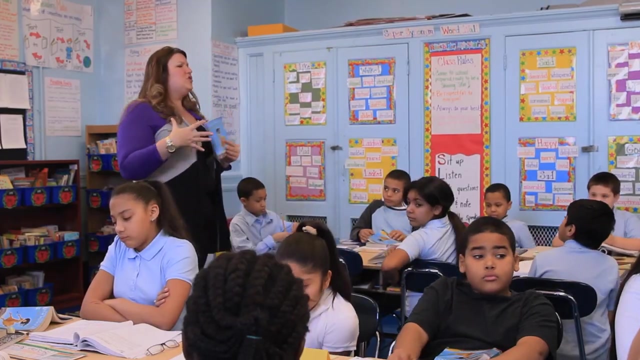 them in the topic of human rights As they read about the threats to the characters human rights. they begin to read articles of the Universal Declaration of Human Rights in order to more deeply understand human rights and how they are being threatened or violated in the novel At all grade. 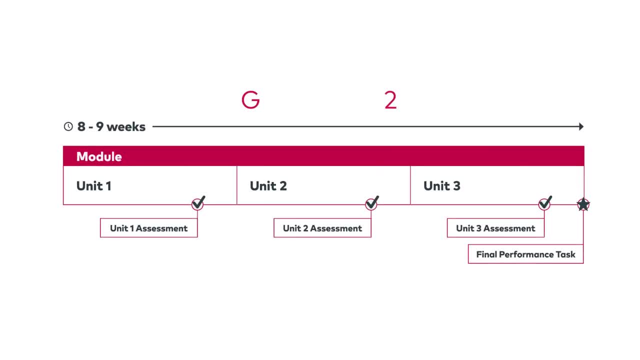 levels. modules include formal assessments: In grades K-2, there is one formal assessment at the end of each unit, for a total of three assessments per module. In grades 3-8, there is a formal assessment at the middle and end of each unit, for a total of six assessments per. 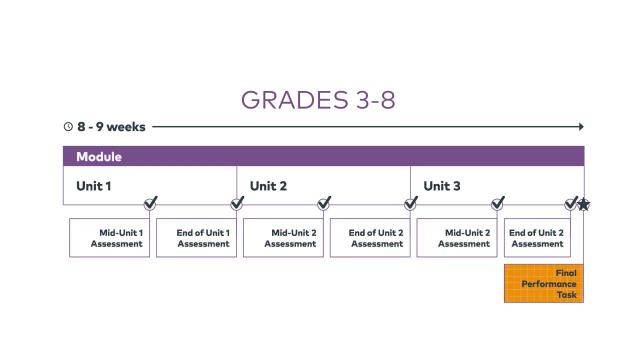 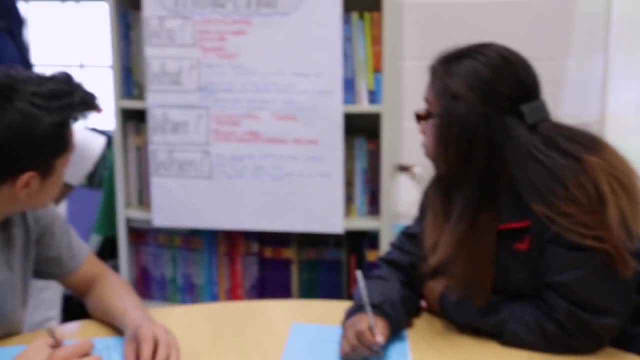 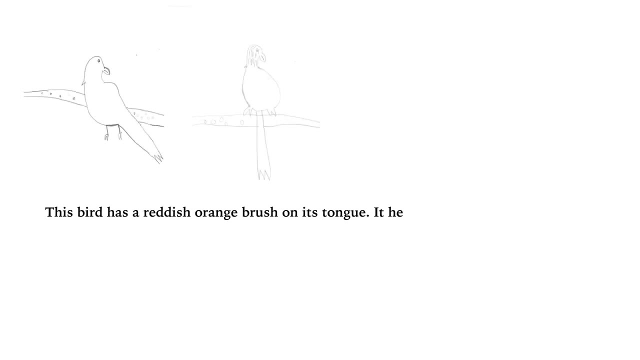 module. Every module in grades K-8 culminates with a final performance task. Throughout unit three of every module, students get support in synthesizing and transferring their literacy skills and content knowledge to an authentic and often collaborative task. The performance task is scaffolded with 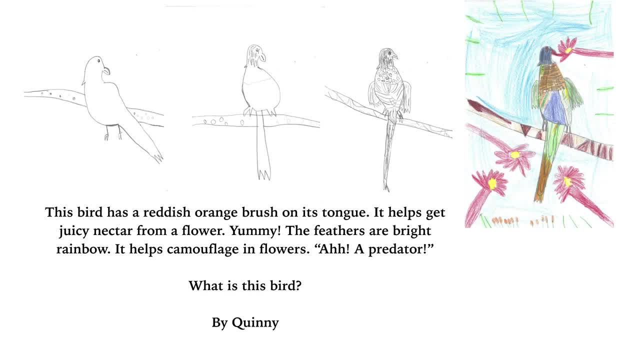 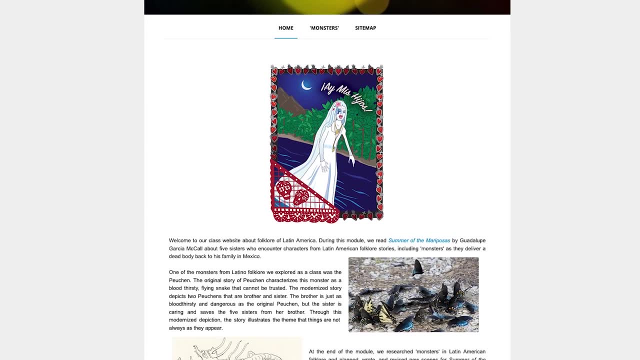 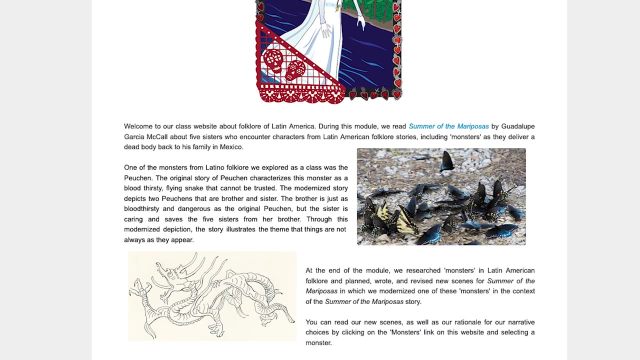 models, drafts, critique and revision, so students produce high quality work. In grade 8, module 1, students learn about Latin American folklore by analyzing narratives and creating their own stories, then analyzing informational essays and writing their own. For their performance tasks, students create a web page for both their narratives and their 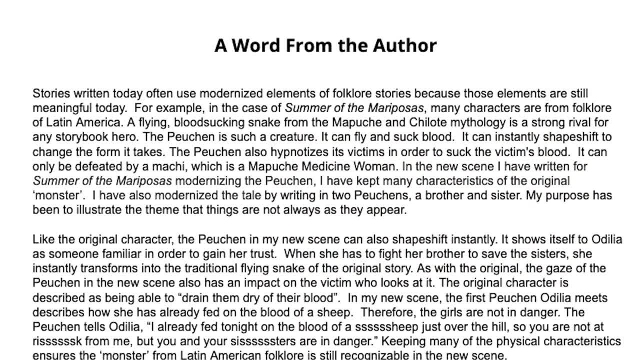 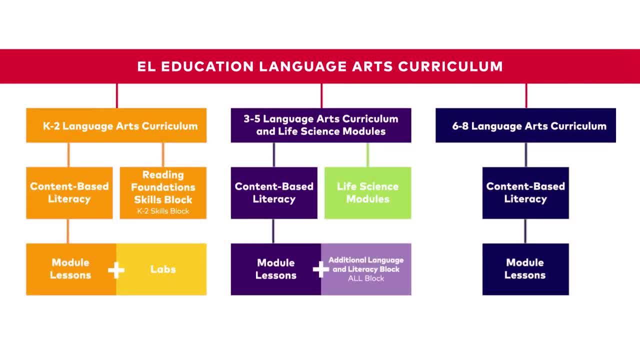 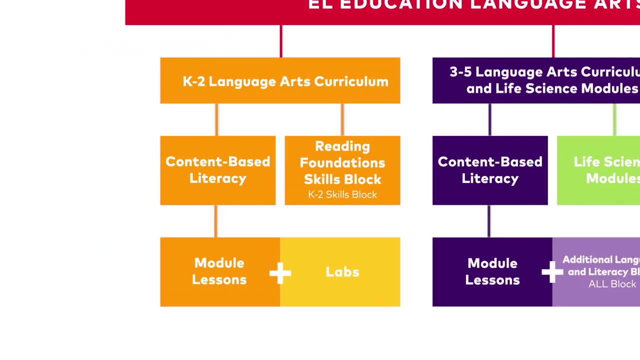 essays, enriching their communities by raising awareness about Latin American folklore. The module lessons are a key component of the curriculum at all grade levels. Grades K-5 have additional instructional blocks to deepen and enhance student learning. The K-2 curriculum offers two hours per day of content-based literacy, The module lessons for one hour and a. 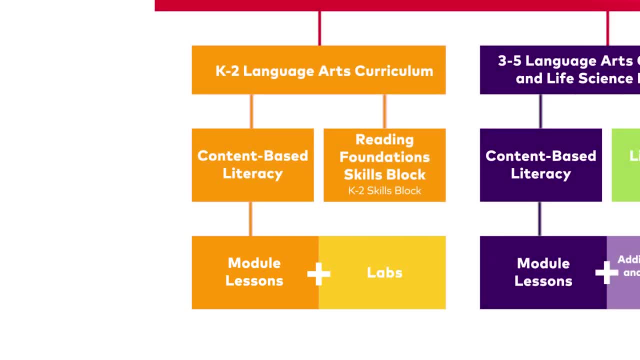 second hour of instruction we call labs, plus one hour of structured phonics we call our reading foundation skills block. Altogether these three hours of curriculum are comprehensive, meaning they explicitly teach, informally assess all college and career ready strands and standards in grades K-2.. Labs: 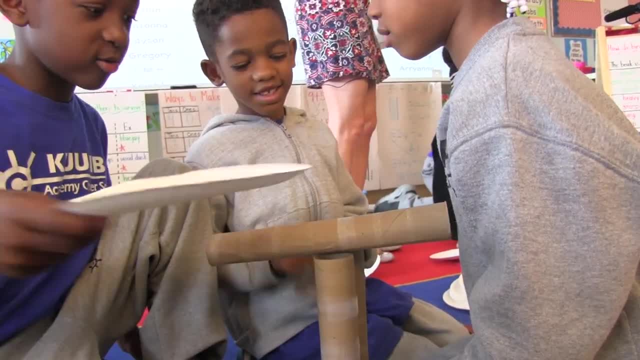 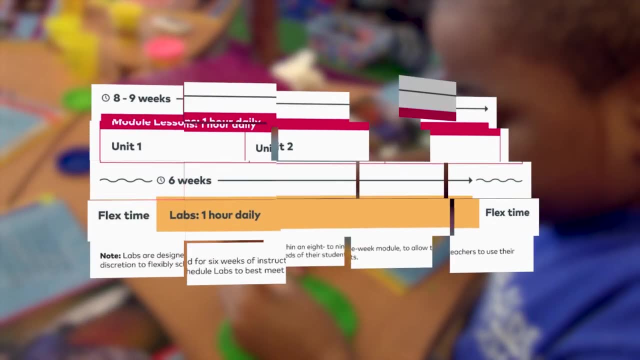 are an important feature of the K-2 curriculum because they support and extend student learning from the module lessons through active learning. The K-2 labs are designed for flexible scheduling of six weeks of hand-to-hand instruction within an eight to nine week module. 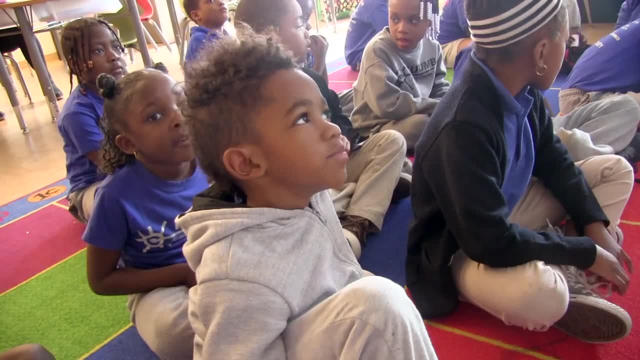 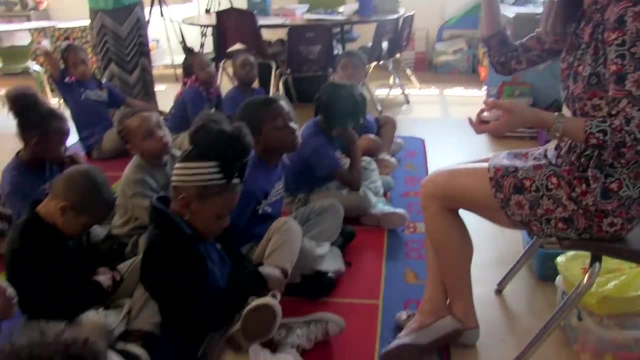 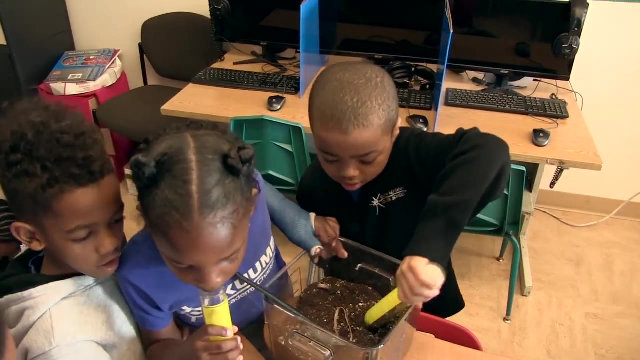 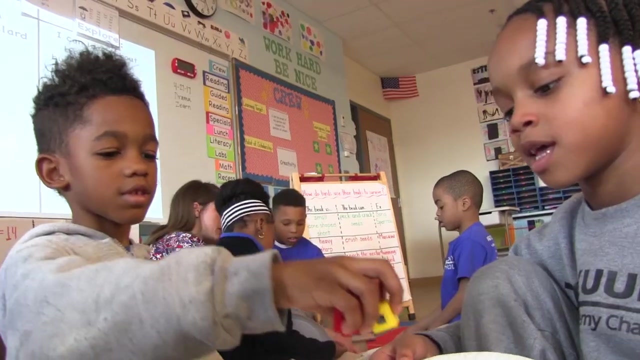 Wow. so that lab where you got to build with those hollow materials really helps us understand how strong a bird's bones are. I've really seen labs excite my kids. it's like ignited this inner fire. there's this like crazy hum that rises up in the room. They're learning through play. they're learning from each other. 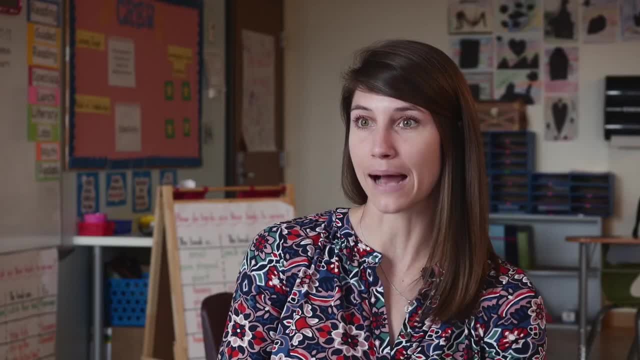 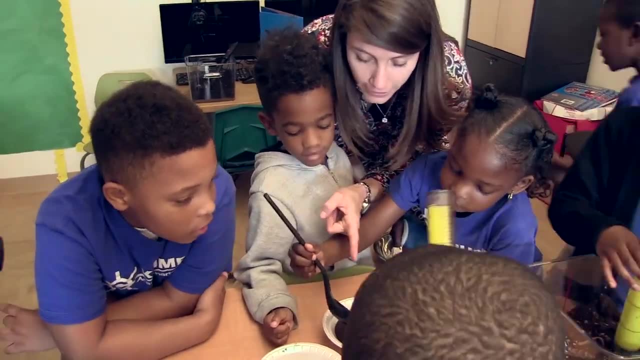 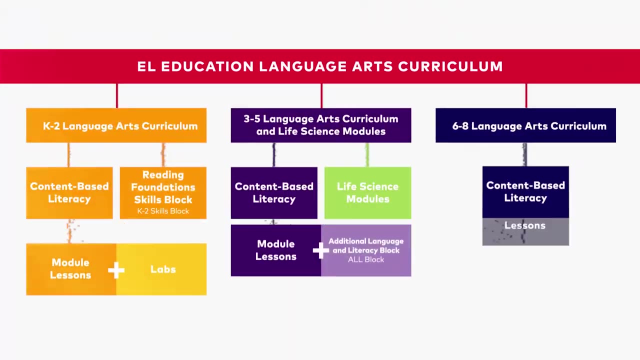 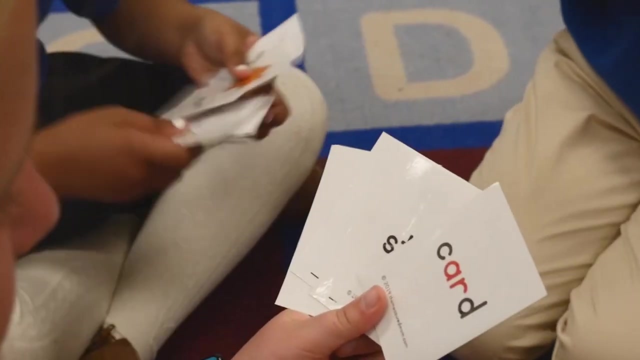 nothing feels overwhelming and there's this sense of joy. Labs are important because they bring joy to the room, joy to the learning and the content. The K-2 reading foundation skills block gives primary students another hour each day of essential structured phonics instruction to help them crack the 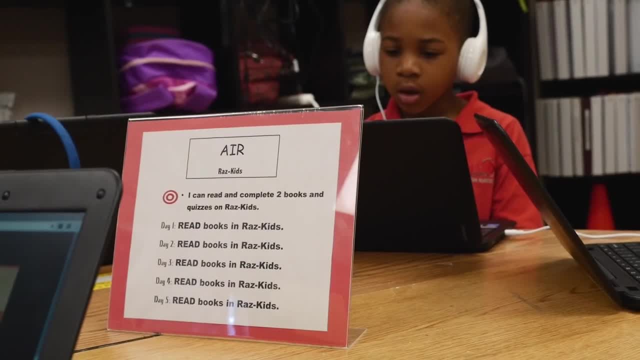 alphabetic code. Like the module lessons, the K-2 reading foundation skills block gives primary students another hour each day of essential structured phonics instruction to help them crack the alphabetic code. Like the module lessons a and the K-2 labs, the K-2 reading foundation skills block is divided into 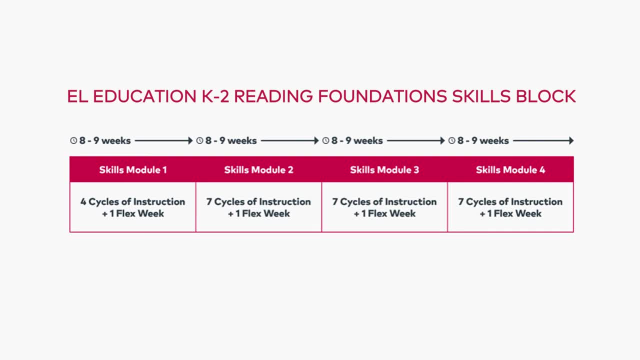 four modules that span a full school year. The first module is six weeks long and the remaining three modules are eight weeks. Each module includes five day cycles, with four days focused on repeated instructional practices and one day on assessment and goal setting, with flex weeks built in to meet the student. 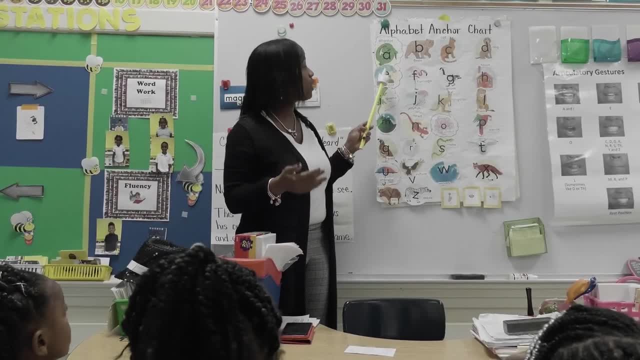 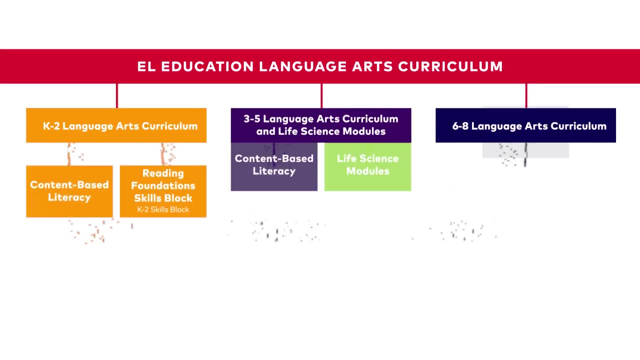 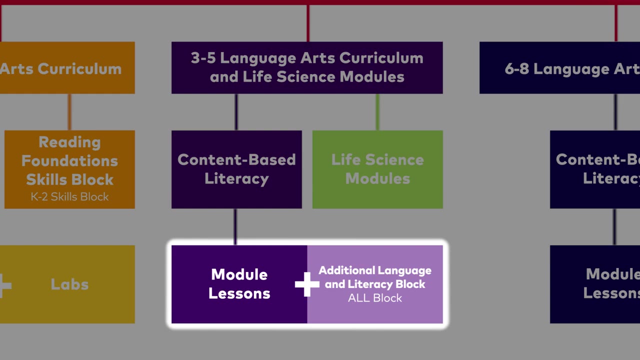 needs. The skills block includes whole class instruction as well as targeted and differentiated small group instruction daily In grades three through five. in addition to the one hour module lessons each day, there's an additional language and literacy block for a second hour of. 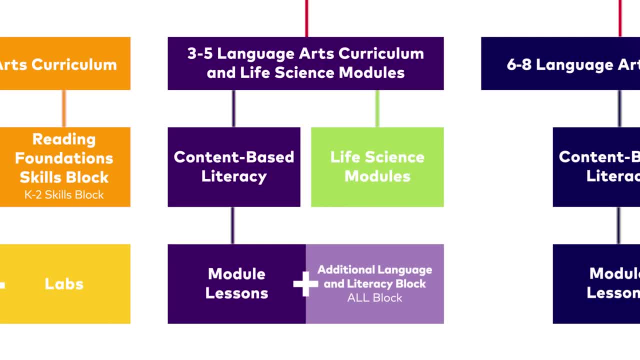 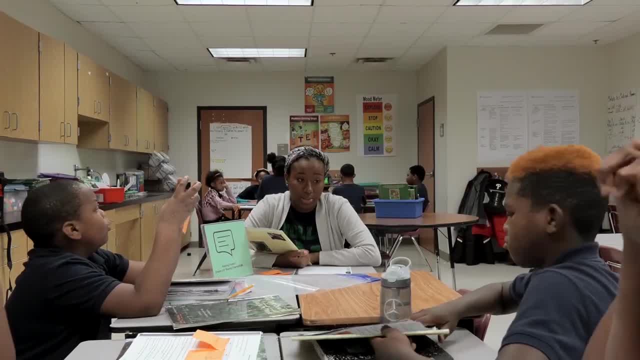 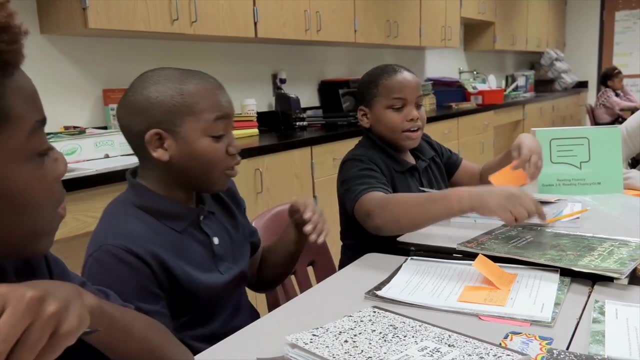 content-based literacy. It's comprised of three units each two weeks in length, with flex time built in. Each unit aligns to the skills, strategies and content taught during the one hour module lesson. The all block responds to upper elementary age students needs for greater independence and mastery. 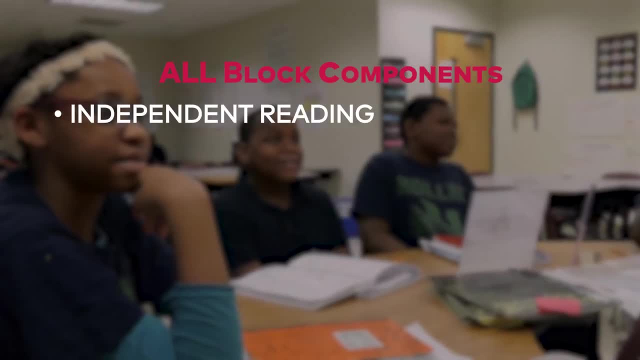 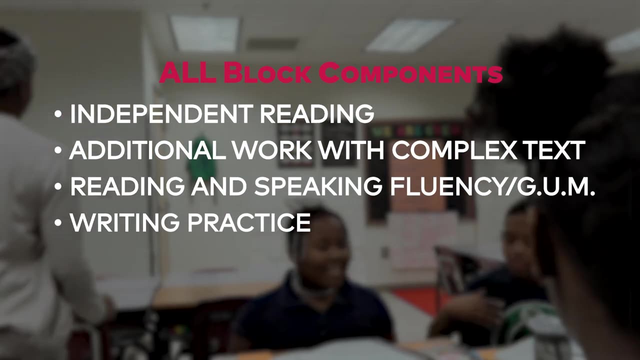 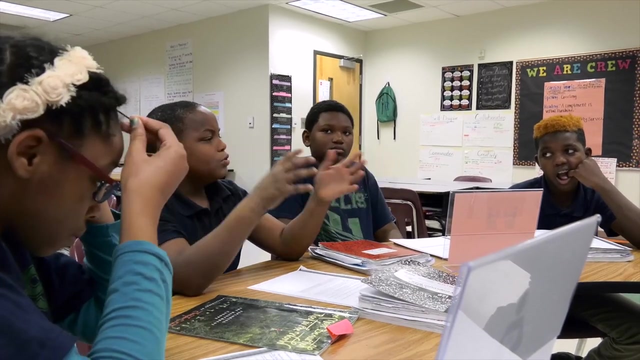 Students rotate in flexible groups to practice independent reading, additional work with complex text reading and speaking, fluency, gum writing practice, word study and vocabulary. I agree with you, but you too. but I disagree with you because he cannot barely keep his eyes open because they're so heavy.